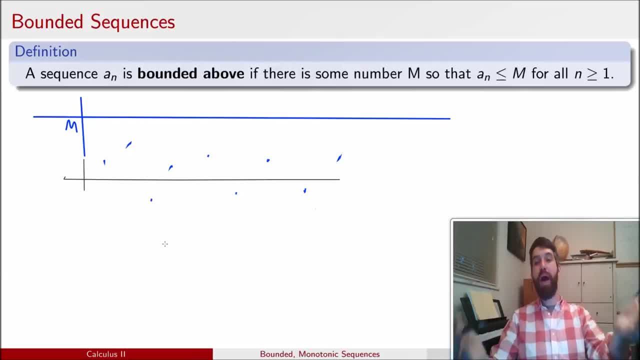 And I might say that my sequence is bounded if it is both bounded from above and bounded from below. The notion of a sequence's increasing is very much analogous to the notion of a function increasing, That is, as I go more to the right, that is, bigger values of n. my function is bigger and bigger and bigger. 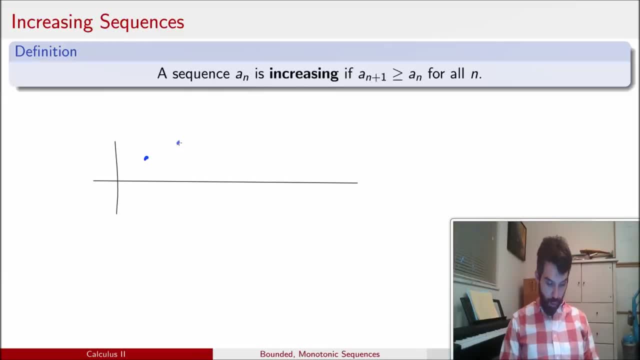 I can visualize this again by plugging in some points and they always get bigger. Maybe sometimes they're exactly equal, but the point is they never go down and they carry on like this. That is an increasing sequence. Likewise I can have a decreasing sequence. It's exactly the same thing. 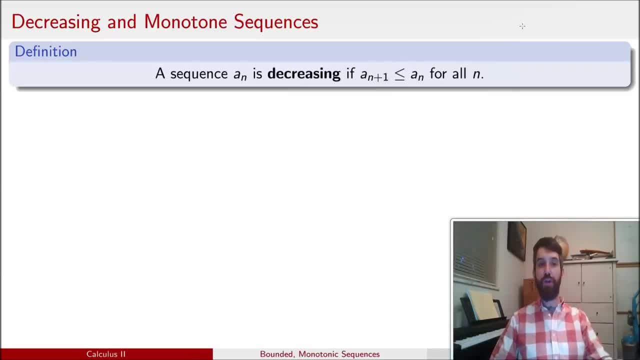 The terms a, n plus 1.. The bigger term, which is a? n plus 1, is always less than the previous terms, And if I have either of those two cases, either increasing or decreasing collectively, those pair of properties are referred to as a sequence being monotone. 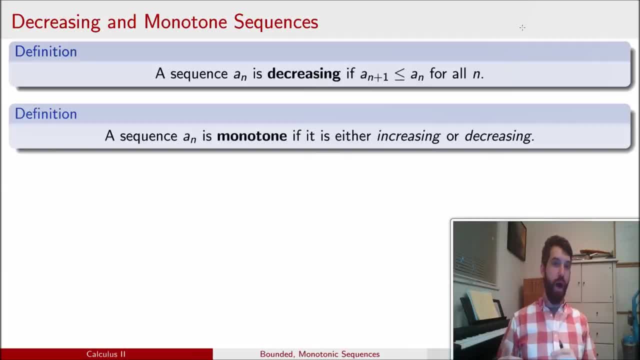 So this is not a sequence that increases for a while and then decreases for a while. That's not what I'm referring to. I'm referring to either the case where it increases forever or the case where it decreases forever. Both of those two cases are collectively referred to as monotone. 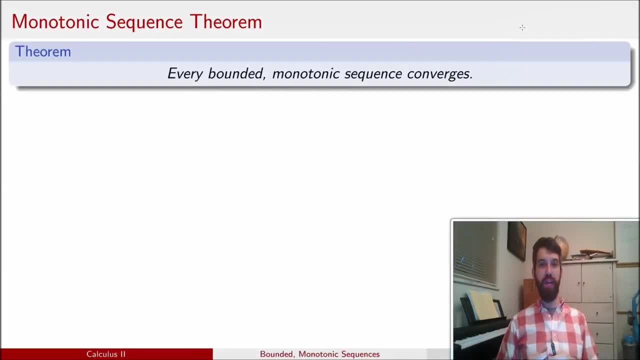 And then we get this very powerful theorem, the monotone sequence theorem, that tells us that both of the properties are true. If our sequence is both bounded and monotone, then we're going to have it being convergent. In other words, we're able to translate the question of does some particular sequence converge? to a test. 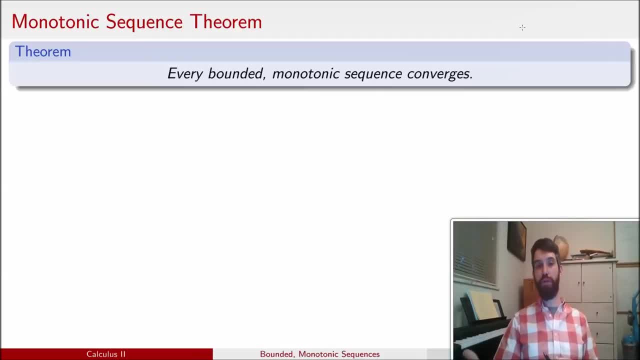 Is it bounded And is it monotone? And if the answer to both of those questions is yes, then it must converge. And note that I'm not claiming what it converges to. We don't know that. I'm merely claiming that it must converge. 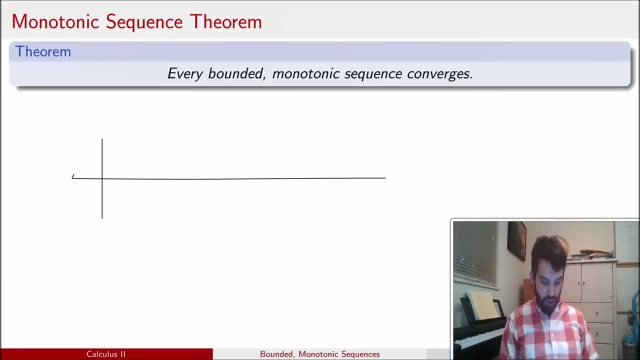 So to illustrate this point, let me first assume that it's bounded And that meant that we had some upper value here that we're going to put in as m, and maybe I'll put some other lower value down in here and I'll call this one n, some negative value. 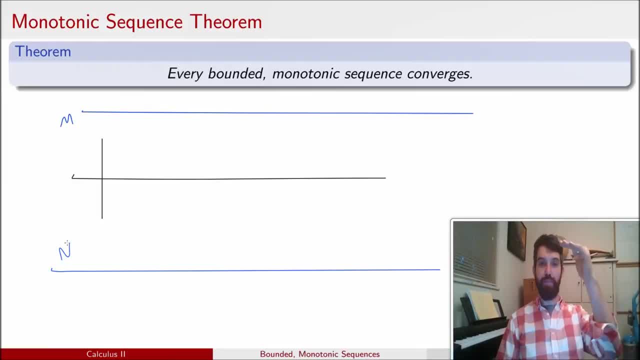 So that was our first condition. Our first condition was that it was bounded. So the sequence, all the terms, have to sort of live in the middle. Now I'm going to assume that it's monotonic. I have a choice of either increase or decrease.